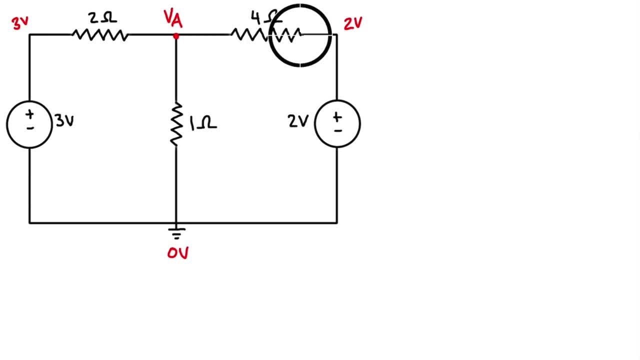 to find this voltage before we can apply Ohm's law to these resistors, because we don't actually know how much current is coming out at the moment. So for nodal analysis, basically the number of nodes with unknown voltages are going to equal the number of equations that we have, And we'll 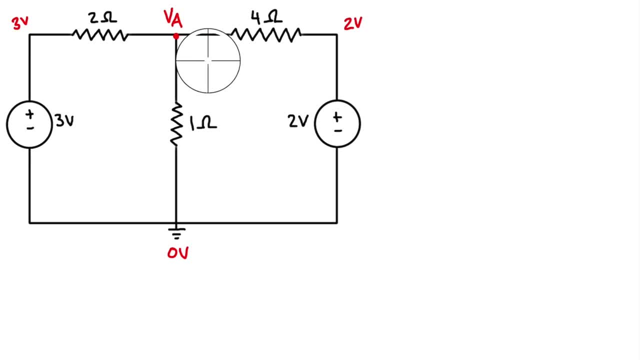 be able to just use back substitution or a matrix or whatever to basically find all of our unknowns, because it will be determinate And the way that we do it is we basically just do KCL at the node. So what we're going to do is we just assume 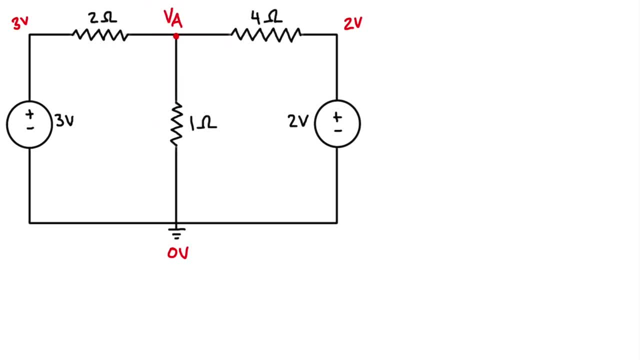 a current coming into and out of the node at all possible branches. So you can just label on the currents that you think there are. It doesn't matter which way they go, But if you think you know it you can try putting them on as you think. So we can call that one I1, we can call this I2.. 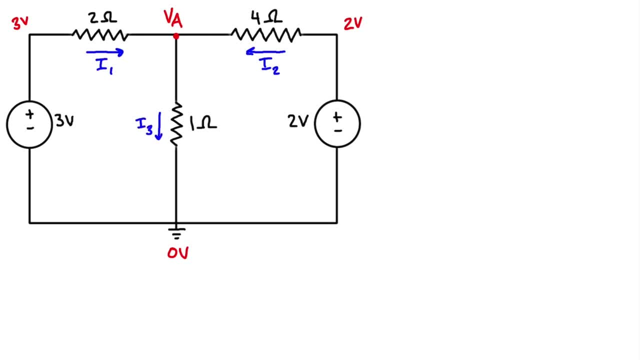 And let's say that we think I3 is going to be going this way, And by assuming a direction of the current through a resistor, that means we're also assuming the polarity of the resistors, because current is always flowing from higher voltage to lower voltage across resistors. That means that 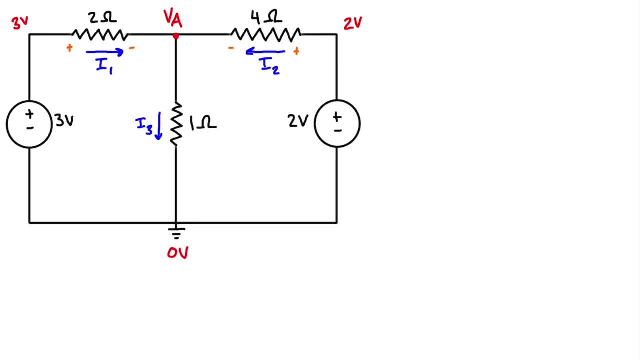 we've assumed the polarity of the resistors And that means that we've assumed the polarity of the polarity like this for all of the resistors. But if you remember, from passive sign convention, the assumption of the polarity doesn't matter, Just if we find that the current to be negative. 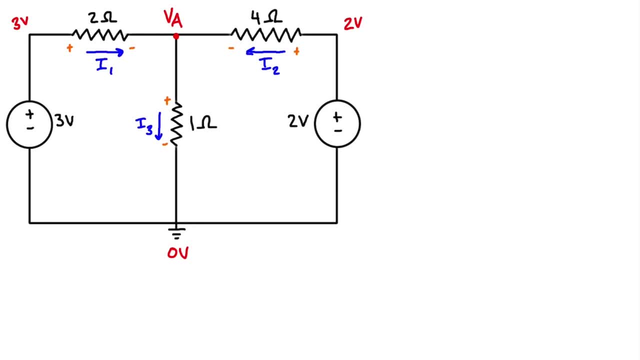 in the resistor, then it just means the polarity was the other way around. So we'll find out if we have these backwards later on in the problem. But yeah, that's basically what's going on here. So we're assuming the VA is lower voltage than three volts and two volts and it's also a higher. 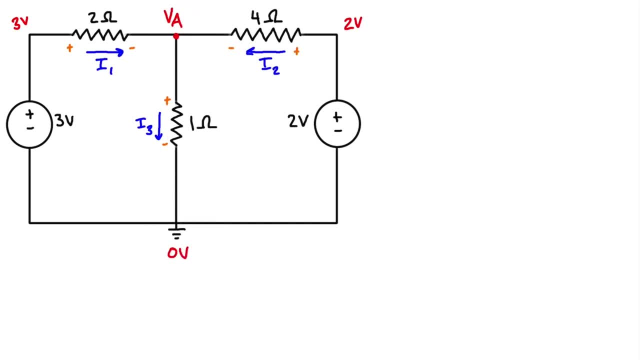 voltage than zero. So now we just write KCL for each unknown node. So in this case there's only one. so we're going to write KCL for A. Just pick a convention and go for it. as for what's positive and negative I like to use, positive is flowing out and negative is flowing in for the currents. 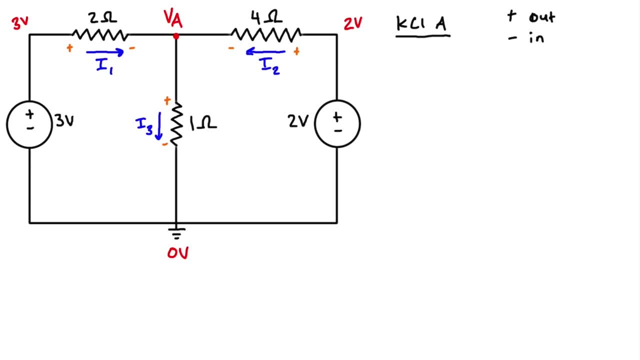 So when we write the expression KCL, basically the sum of currents has to equal to zero. So I1 and I2 are flowing in, so they're going to be negative, And I3 is positive, so it's flowing out. So let's maybe write that one first. So we have. so it looks a bit nicer. we have I3. 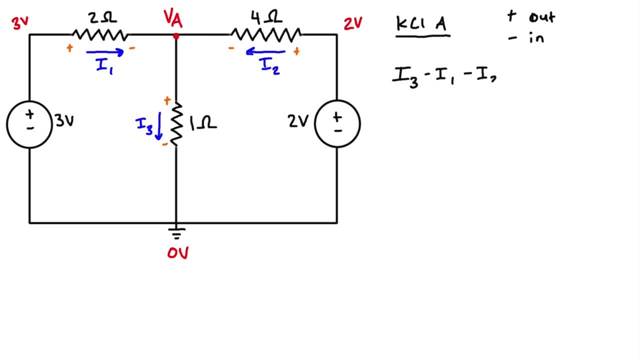 minus I1 minus I2 is equal to zero. This is the expression for Kirchhoff's current law for the whole node that we're calling A. Now, if you remember Ohm's law, we have: V equals IR and we can rearrange this to be: I is equal to voltage over resistance. So we just need: 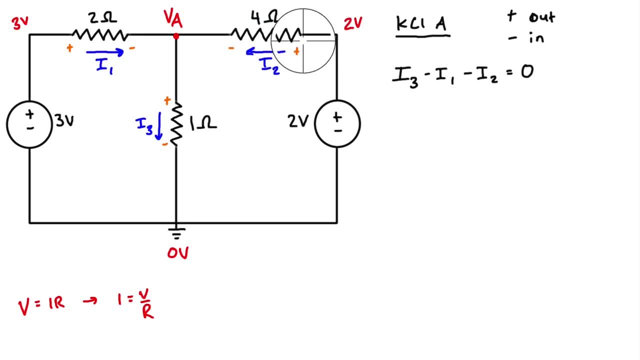 to get these in terms of the voltage and resistance, and we actually can write those. So let's start with I3.. The voltage across this resistor is VA minus zero, because we've assumed that VA is higher. So when we subtract the lower one, 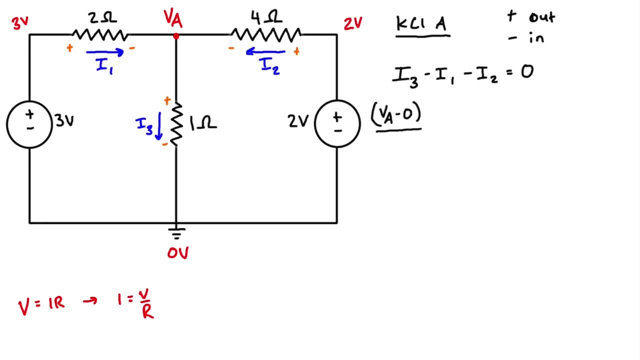 this is going to be the voltage drop. And then we divide this by the resistance, which is one ohm. Then for this resistor, that I1 is flowing through the voltage, first of all, we subtract this one and the voltage is three volts minus VA. Again, we've assumed that the current is going this way. 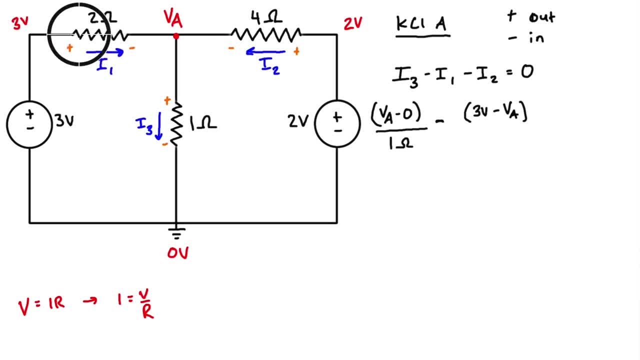 so that this is the higher voltage. So the difference between them is the bigger one minus the smaller one. So that's why we have three volts minus VA, And then we just divide that by the resistance, which is two ohms, And then for the other resistor we do the same thing. So the voltage 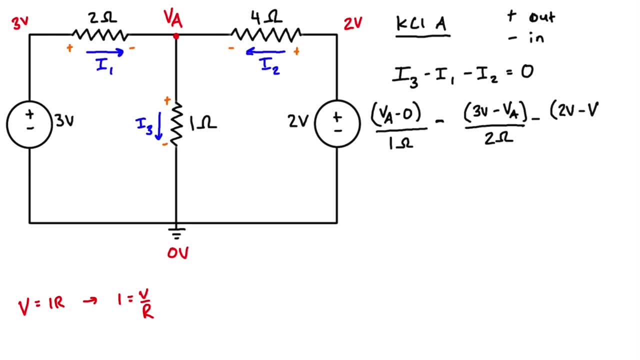 drop across the resistor is two volts minus VA. Again, we're assuming two volts to be bigger. so we're subtracting AVA, which is the smaller one, over the resistance, which is four ohms, And I ran out of space. but that's all equal to zero. 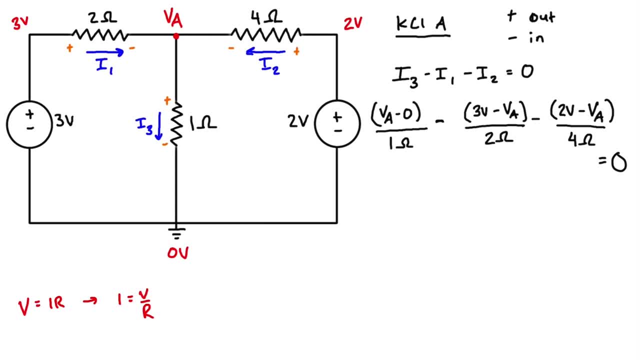 Okay, so we just want to simplify this. You can see there's only one unknown in here, So one unknown and one equation. that's pretty easy. Let's multiply everything by four to get rid of these numbers on the denominator. So we have four, four and four, And then we can just divide this. 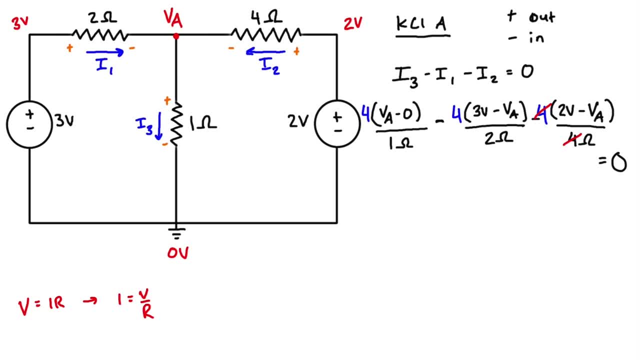 basically that's going to be nothing. This four and this two are going to cancel, So we have minus two and then this four divided by the one, that's basically just the one. So let's maybe write this a little bit cleaner. We have four times VA minus two times three times VA. 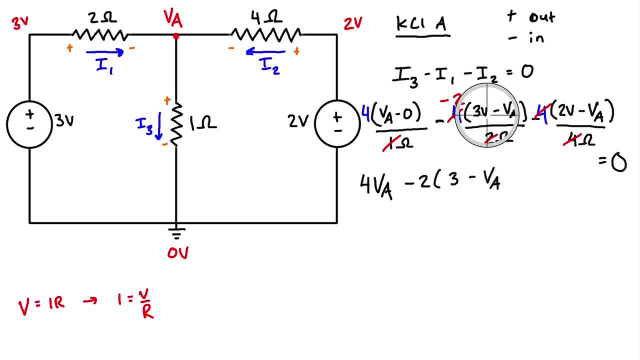 I'm going to drop the units of ohms and volts because it gets confusing when you have the V here for volts and VA for the unknown variable. So basically, each term is going to be in units of volts over ohms, which is in units of amps. the whole term is: 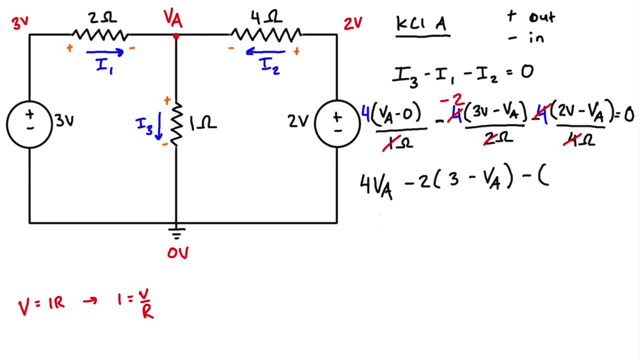 So we can close that bracket and then we just have minus two minus VA is equal to zero. So we can simplify this a little bit and we get four VA minus six plus two VA minus two plus VA is equal to zero. So basically we get seven: VA is equal to eight. 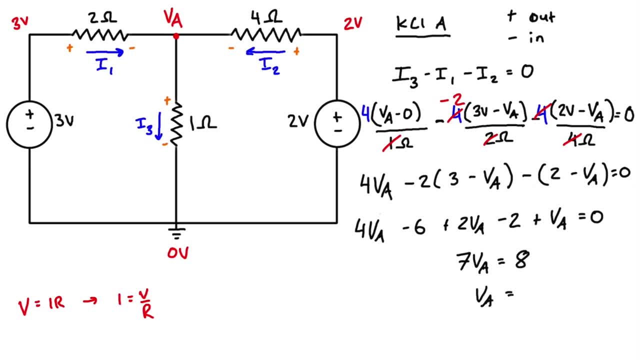 and then we can just rearrange for VA and find that this is about 1.143 volts. So yeah, we found the voltage now of this node, but it's probably also useful, or requested of you, to find the currents that are flowing through where the voltage drops across these resistors. So let's. 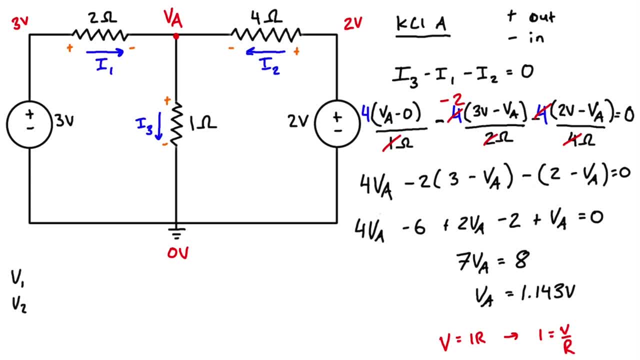 quickly do that. So we have V1,, V2, and V3 for the voltage drops across the resistors corresponding to each of the same currents: one, two and three. So the voltage drop across the first resistor is three volts minus 1.143 volts and that is just equal to 1.857 volts. 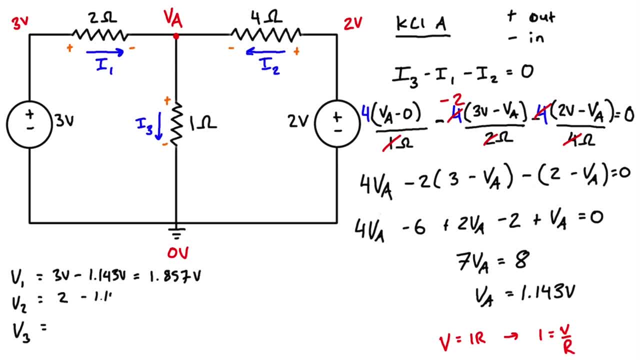 For V2, we have two minus 1.143.. And that's equal to 0.857 volts. And then for V3, we just have 1.143 minus 0. So that's equal to 1.143 volts. 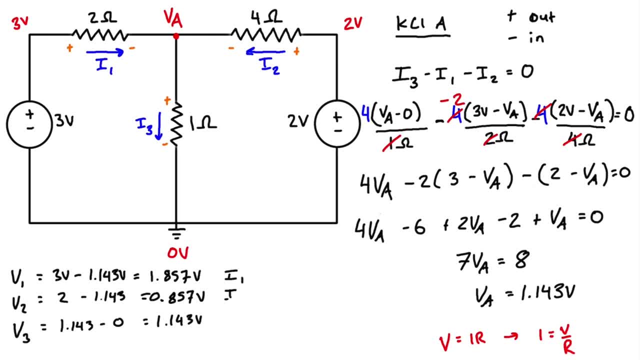 And then we want to solve for the currents. for each of those We have I1,, I2, and I3.. Well, the current again is just equal to V over R, So we have 1.857 volts over 2 ohms. 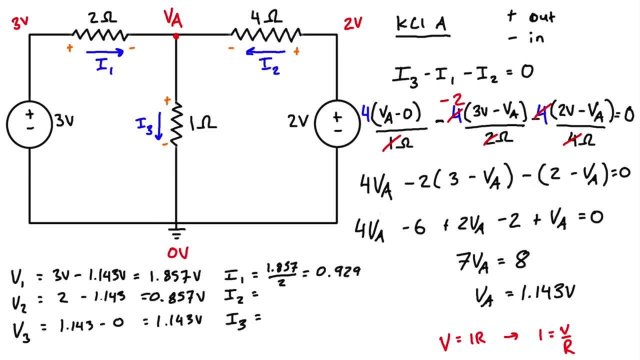 And that gives us a value of 0.929 amps. And then I2 is just 0.857 volts over 4 ohms, And that gives us 0.214.. And then for I3, we have 1.143 volts divided by 1 ohm. 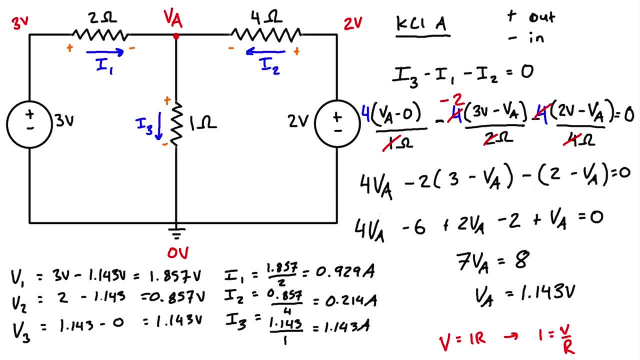 And that gives us 1.143 amps. And just to double check, when we look at this we have for KCL Kirchhoff's Current Law at the node we have I3 minus I1 minus I2.. So basically the sum of currents flowing in.